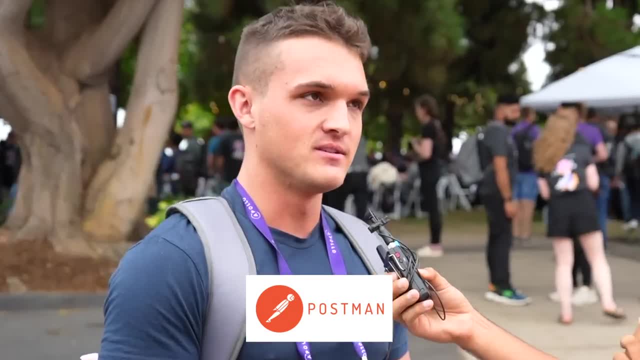 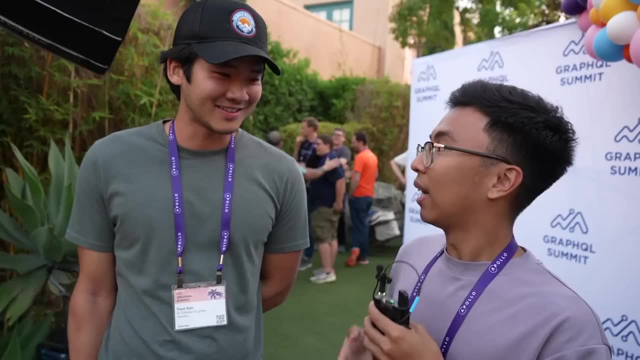 How much money do you make as a developer? Um, ooh, I mean, Yeah, I make around. I would say My first job, my salary, was Today. me and my friend are at GraphQL Summit asking these developers how much money they make. 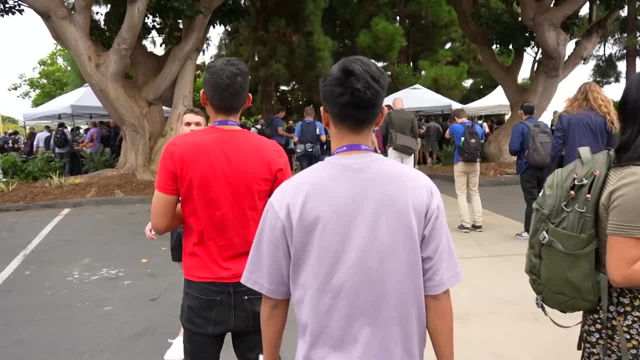 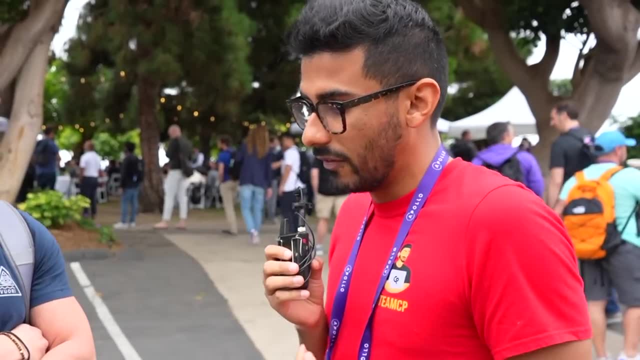 And wait till you get the end, because the numbers get crazy. Yo, what's up, bro? Oh bro, Postman. Yeah, Every developer on our channel knows about Postman. So what would be one piece of advice for somebody who's looking to get their first job? 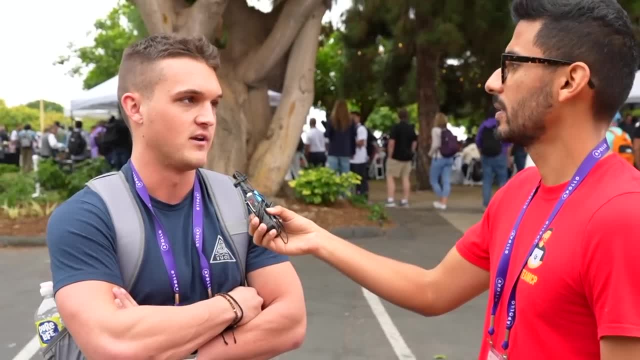 Yeah, I don't have a degree. I'm from Oklahoma City, so there's not a whole lot of tech there. So what I really did is I really contributed to a lot of open source projects. I didn't actually apply for my Postman job. 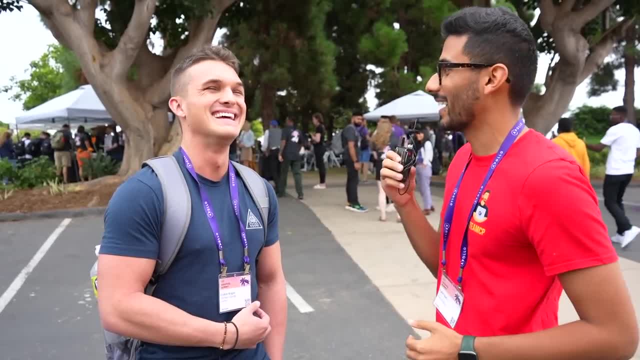 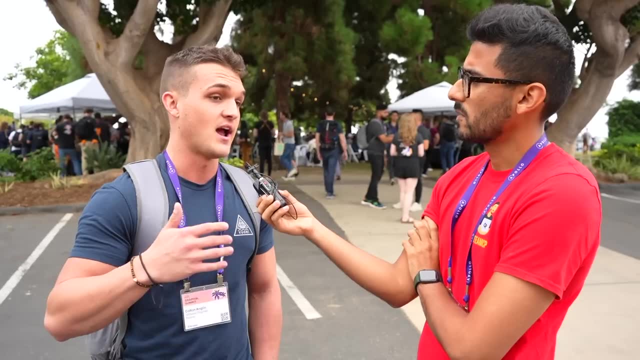 They reached out to me So um, So how much money do you make as a developer? Um, I make six figures and that's as an SE1.. So that's like entry-level software engineer and I have great benefits. 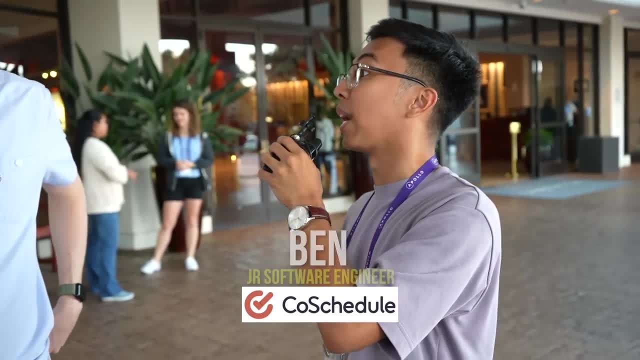 So we're here with Ben, If you're comfortable sharing. how much do you make as a developer now? Ooh, I'll give you a range, boys, I'm not gonna give you it all. Uh, 100 to 110.. 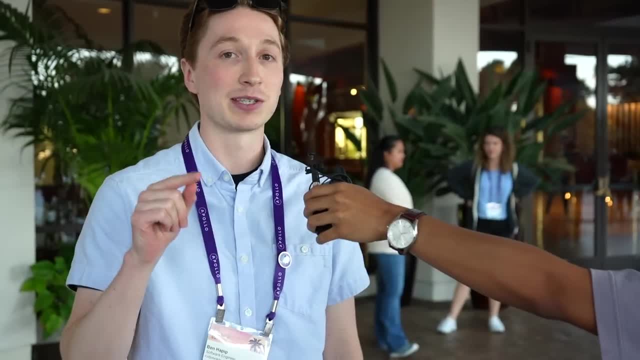 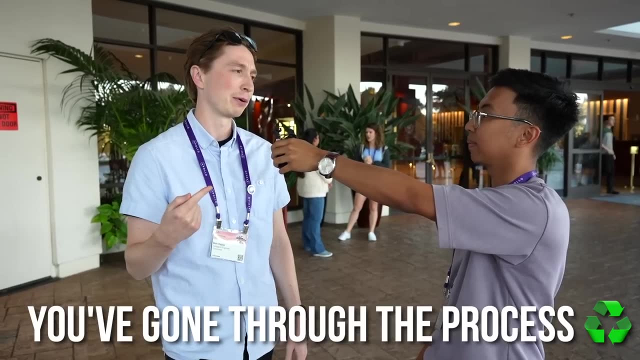 So I got an internship actually in college. I should say that That's a major key: You get at least like a three-month internship. That'll negate any sort of experience because then, like you've gone through the process at that point. 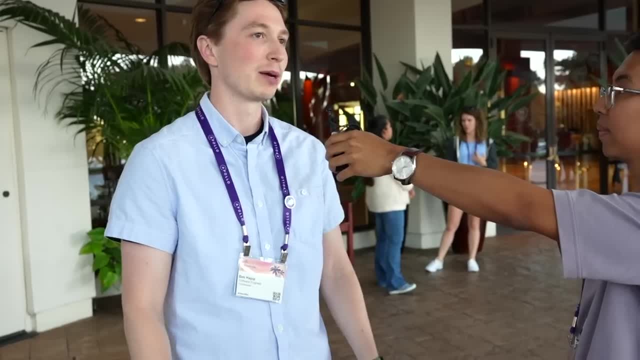 You know you've gone through the software development lifecycle. Once you've done that, most jobs are like: all right, you're good to go. My name is Camille. Uh, I'm 24.. Uh, I'm a front-end software engineer. 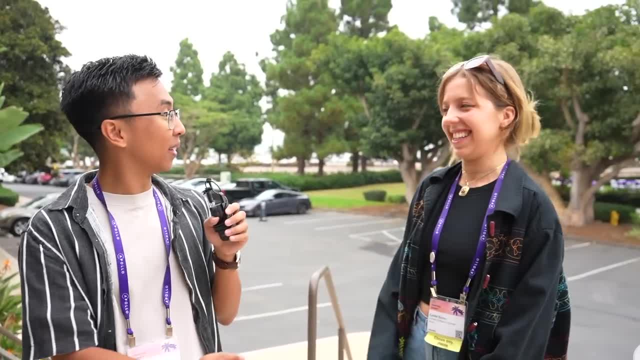 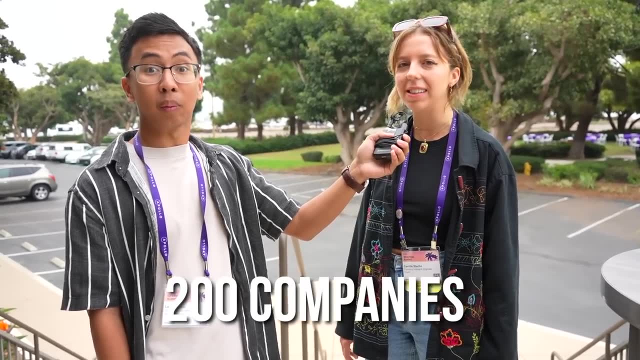 I work at Peloton in New York City. Wait, so your first job was with Peloton? Yes, my first job was with Peloton. Wow, amazing. And how did you go about getting your first job? Oof? I applied to probably 200 companies. 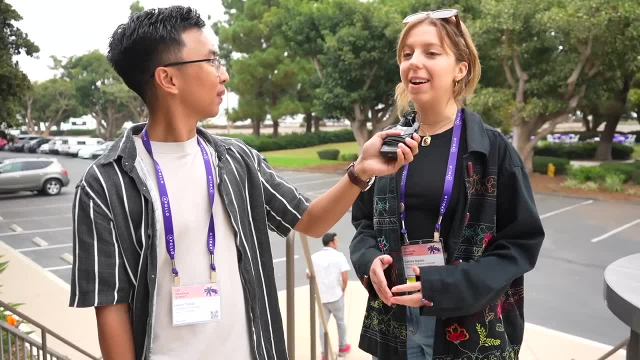 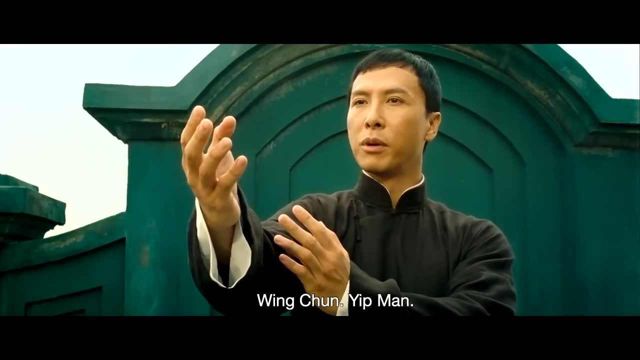 Wow, Maybe like 10 people will be like: hey, Never forget that people want to refer you because they get referral bonuses. If you don't mind sharing, how much did you make on your first developer job, Yongchun? 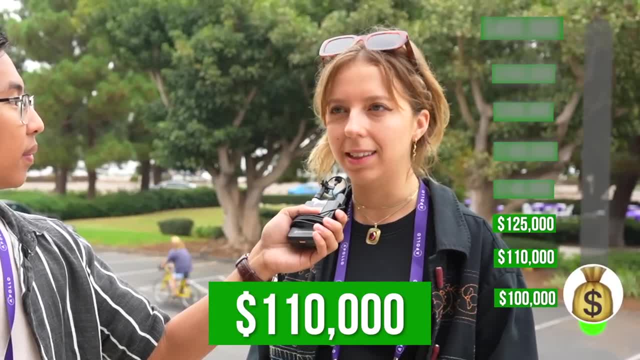 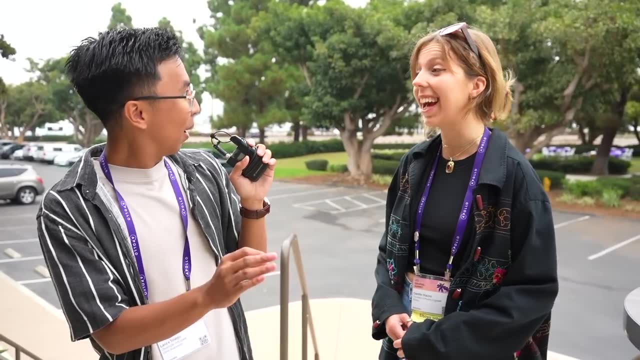 Uh, so my first job. my salary was 110.. I had a 15K signing bonus- Amazing- And my equity was. You got equity as well. Wow, that's awesome. Yeah, Wow, Peloton, It used to be worth a lot more. We've had an amazing time meeting people. One piece of advice: If you thought $125,000 is a lot, then you'll be surprised to see what some of these developers are getting paid at the biggest companies. The thing is, developers are often shy about their salaries. 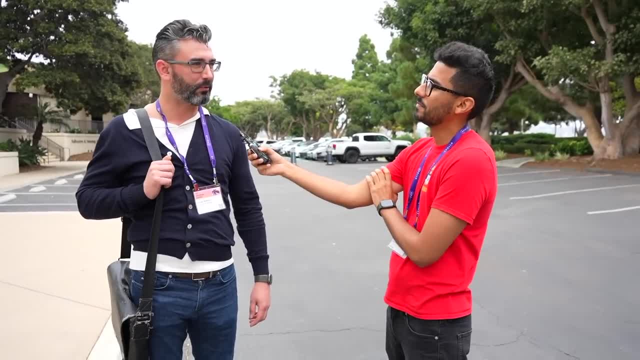 How much money do you make as a software engineer? Uh, I will not reveal that. I'm not comfortable sharing that. Uh, I don't want to answer that. Uh, no, I can't do that, Sorry, No worries. 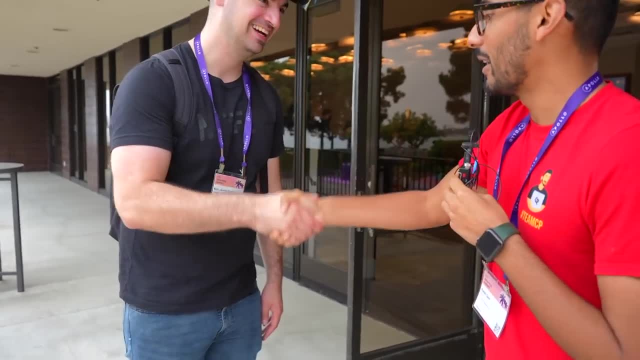 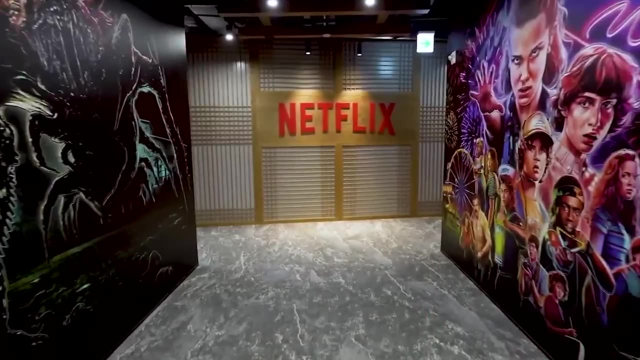 Will we find people willing to share? Yo, that is awesome. Nice to meet you, Mark. What's it like working at Netflix? Ooh, uh, I mean it's great, It's fun. Uh, it's a big company, but you get a lot of freedom. 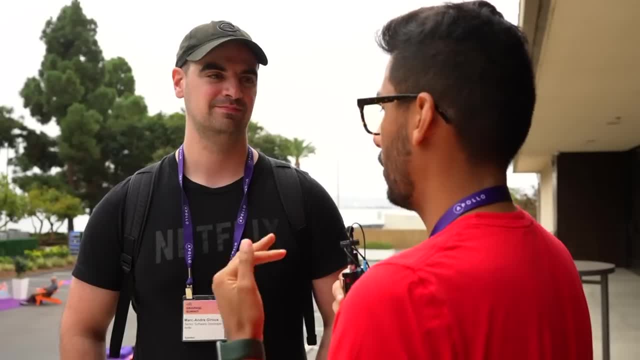 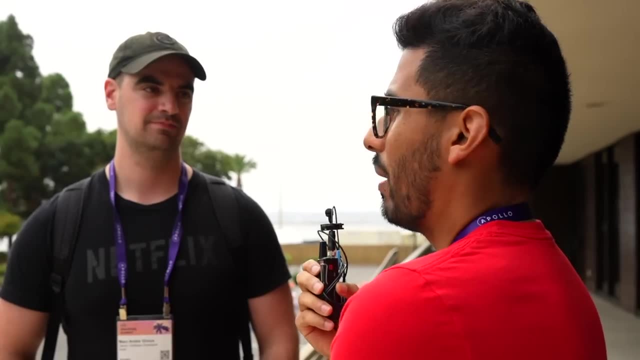 I've talked to people and they're like: Hey, even over sometimes a senior developer that prefers somebody who's maybe junior and but is like really hungry, but they don't have the greatest amount of experience. Is it possible they could work at a company like Netflix? 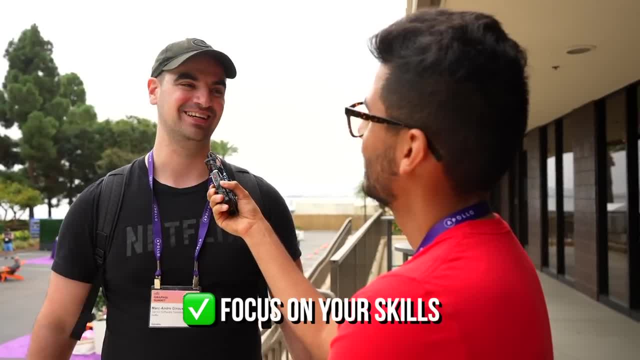 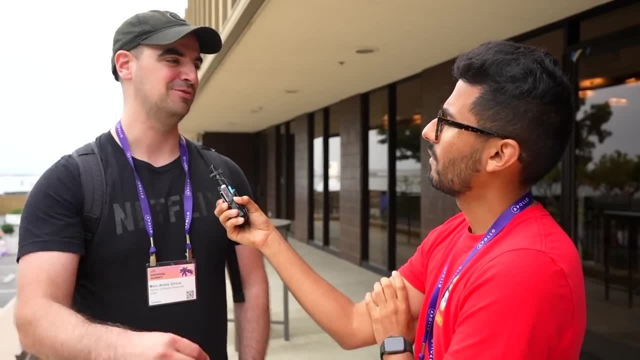 I mean, I think it's possible. I think it depends Like: keep focusing on your skills. Skills are really truly what matters. Trying to show your skills through other means because clearly you don't have like experience. So understanding what you use we often use like frameworks and libraries. actually reading a lot of code, digging into those libraries, I think is super important. 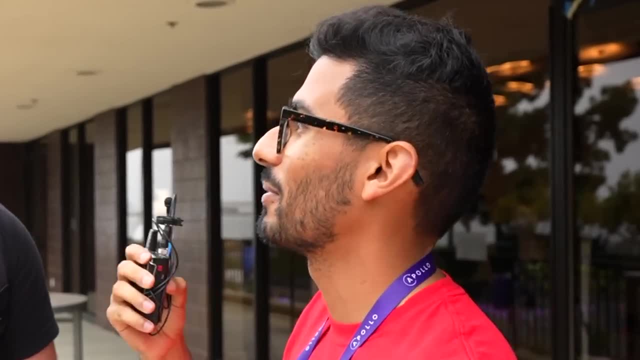 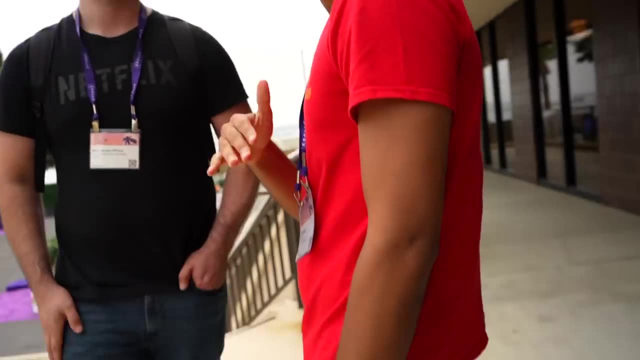 So if you're comfortable sharing, well, how much do you make as a software developer? I don't think I'm comfortable sharing. Got it Well. thank you so much, Mark. Appreciate it Now. that was unfortunate, but these next developers are earning multiple six figures. 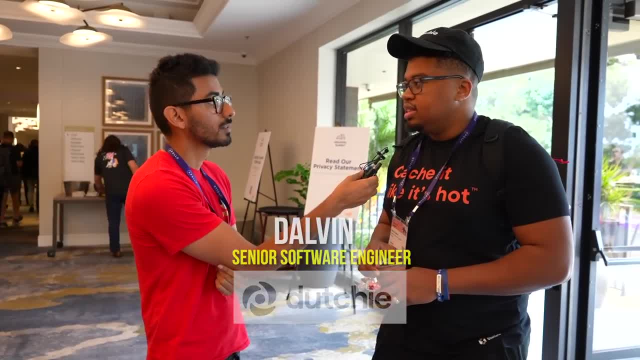 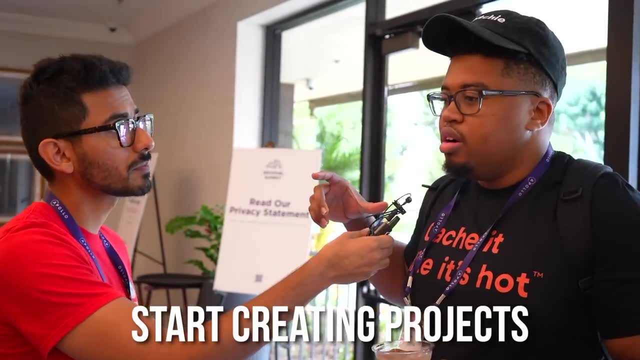 I'm here with Dalvin, So my advice for somebody who wants to get into tech for the first time would be: start trying to learn on YouTube. You don't have to go to a bootcamp or pay money if you don't want to start creating projects that you're interested in doing, stuff that you like. 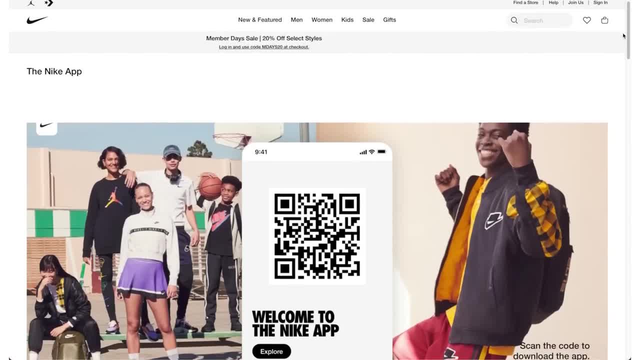 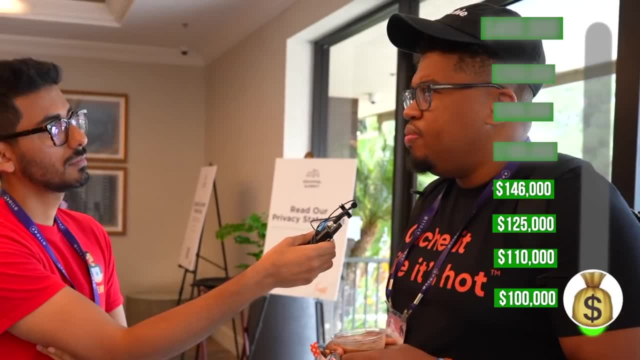 If I'm into sneakers, I'm going to try to make the Nike app again and put it on my portfolio and resume. Are you willing to say how much you make right now? Yeah, So currently I make 146.. Damn, That is amazing. 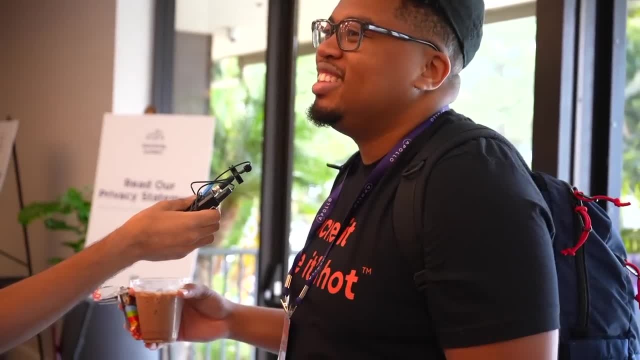 It's basically fake it till you make it. Yeah, That's like my best advice. So I'm here with Trent, I guess. tell us about yourself, Like, what do you do? Sure, I'm a full stack engineer at Glassdoor. 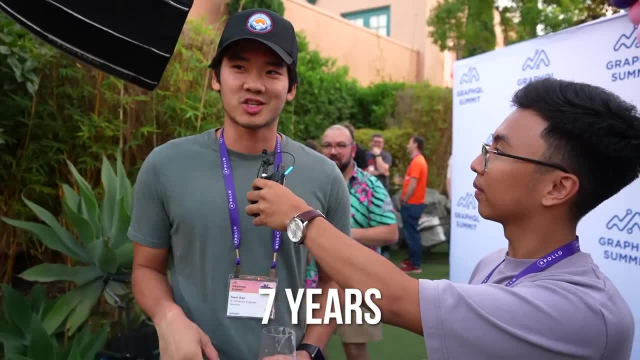 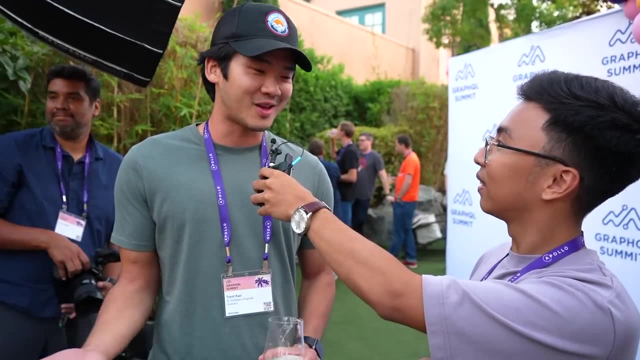 I've been doing this for about seven years now And I actually in college I was a pre-med major and switched to this last minute And it turned out to be a pretty good decision. I never would have thought I would be here at a tech conference. 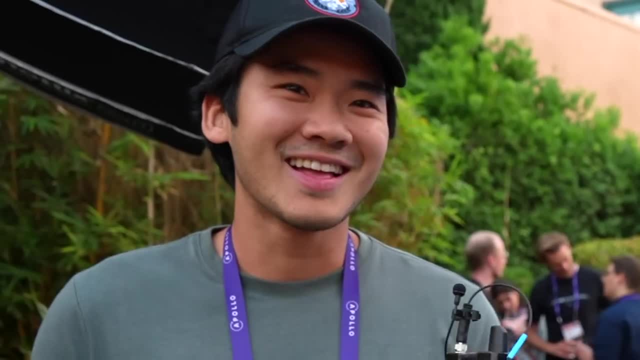 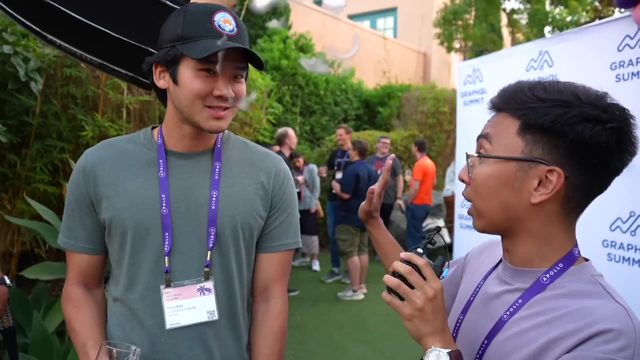 And here I am. Do you want to share how much you made at your first CS job? Sure, I made. it was 70 grand. 70 grand In Chicago, In Chicago. And how about now? What do you want to give a range of like how much you're making? 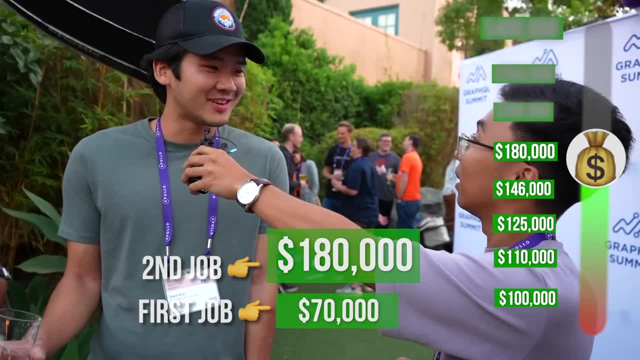 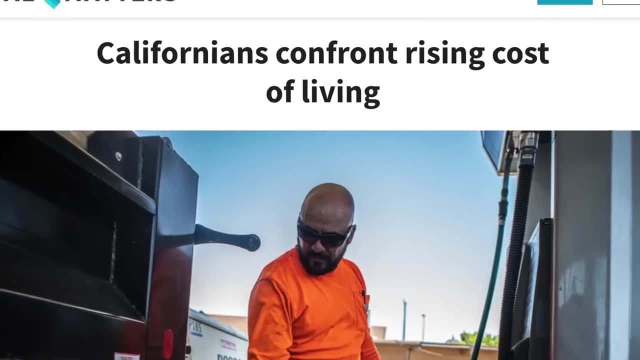 I think I make 180 grand now after six, seven years. Congratulations. Yeah, That's amazing. Yeah, Which is nothing for you know, California, but Chicago, The cost of living, the cost of living in California. I'm here with Alex guys. 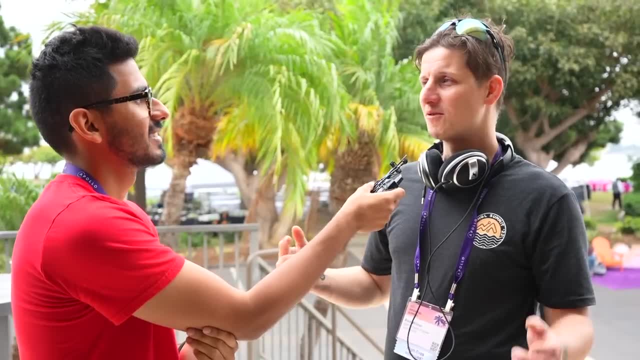 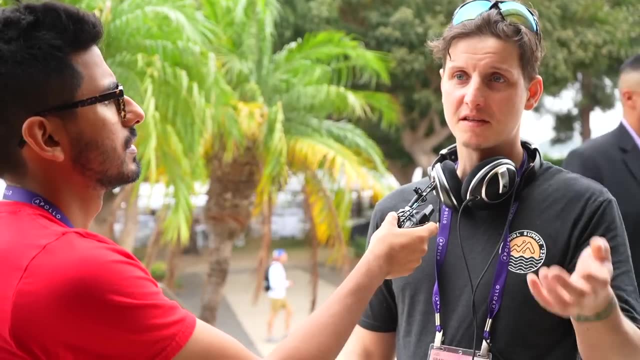 So I'm a DJ, right, I needed to make an app to help me organize my music. I didn't know how to code anything, But the thing that I learned through that process was that I didn't hate it. Yeah, Because one thing that I see a lot of newcomers come in like they see the price tag and then they get a month into the job. 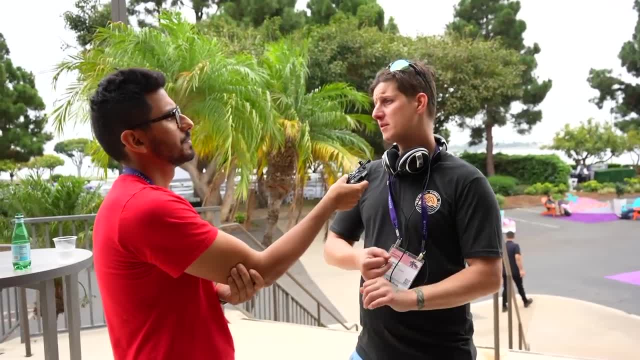 Yeah. And then they get a month into the job And then they realize like, oh, this is what I want. And then they realize I don't really like coding that much. Join a community, Try building something. Figure out that process for yourself. And if you like it, then you should be good to go. How much money do you make as a software developer? 2013,, I started at 40 grand. After a year there, they bumped me to 75.. By the end of 2018, I was a lead dev for 130. And then I'm in that like range, like 200-ish. That is amazing Man, I would say. so I've hired a lot of junior devs. If you're like totally fresh, you're probably looking in the 60, 70 range, which I think is still really good these days. 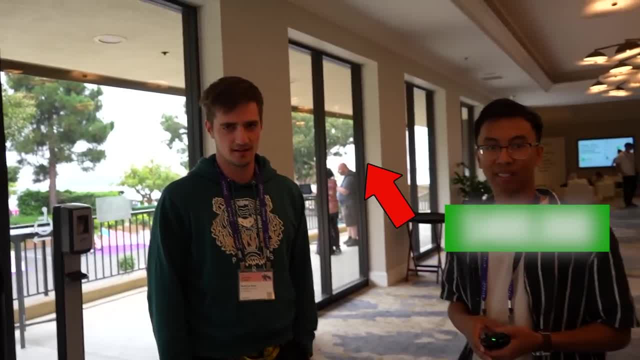 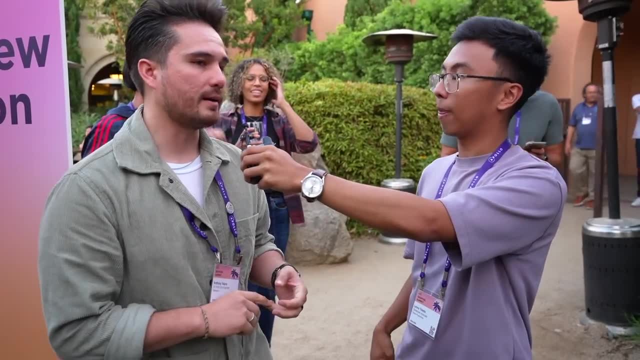 If you thought $200,000 was a lot. these next two developers, These developers are paid crazy, All right, so I'm here with Anthony. Tell us about yourself. Went to college for computer science. Ended up dropping out and just going self-learning route. 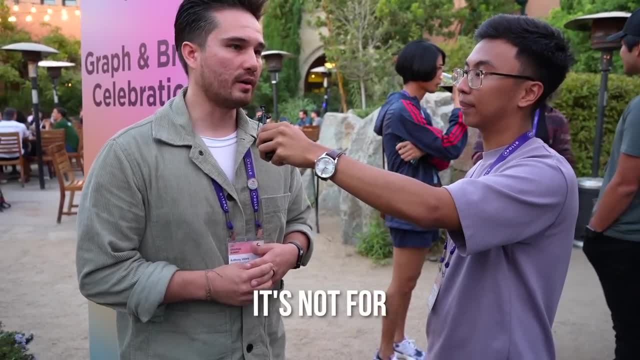 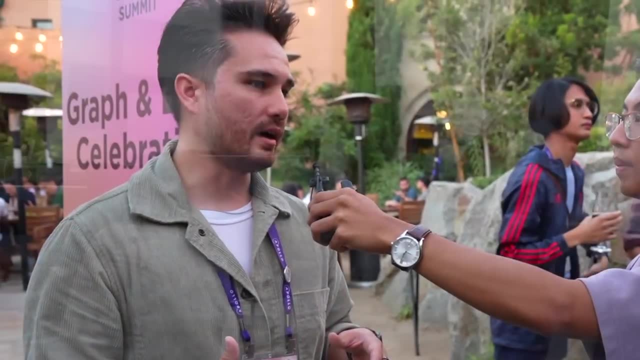 Anyone can get into this career path. It's not like for intelligent people. I've seen people who have worked their whole lives in like the service industry Go into like a boot camp Or go into like a self-learning path. 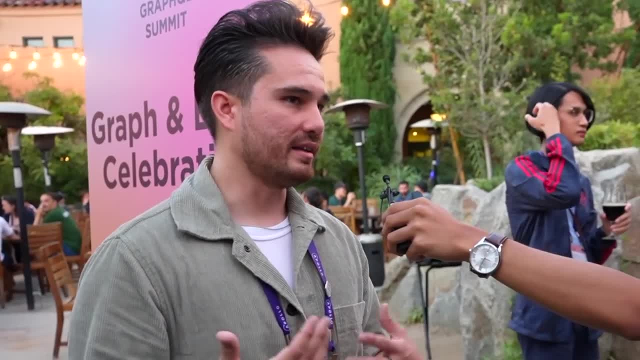 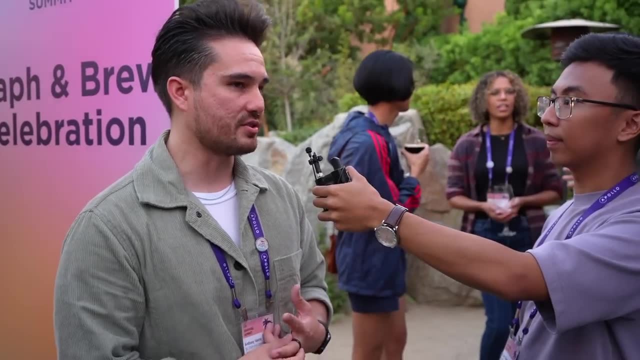 And come out making two to three times the amount of money that they were And being two to three times Happier in their role. It's for everyone. But I ended up getting a job as a junior web developer And then, from there, just improving my skills. And I made $17,000 an hour. It was like $30,000 a year. Amazing, And if you don't mind sharing like a range of how much do you make now? Yeah, I make around $250,000 a year. 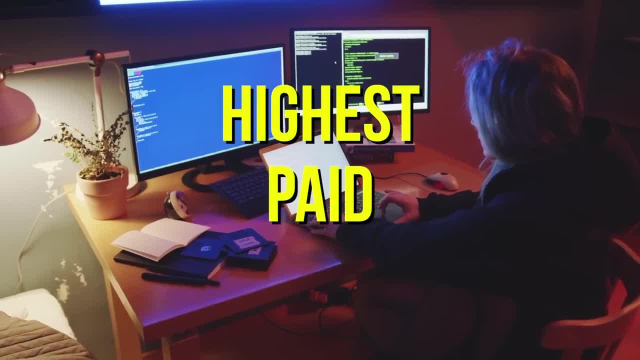 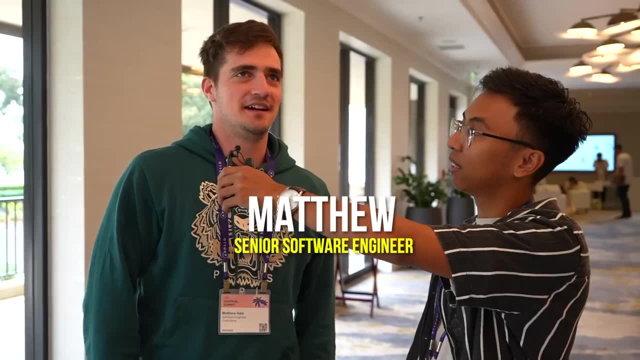 Yeah, This next developer is among the highest paid developers on Earth, And this is how we got here. What's up, guys? I'm here with Matthew. Tell us a little bit about yourself. I am a developer at Credit Karma. I have been for the past four-ish years. 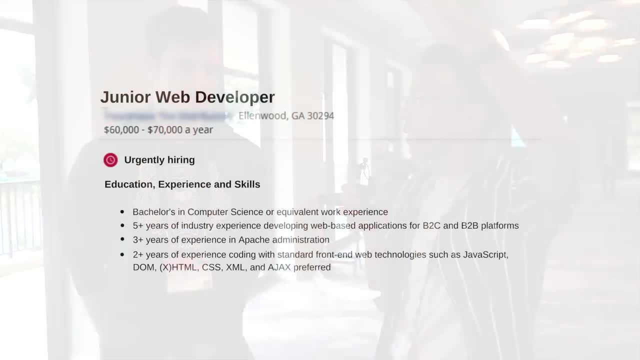 Since, like 2018.. Right, We have a lot of developers. When they look at the job posting it says like Hey, we need like one year to five years of experience. So, like, how would you be your advice for that? 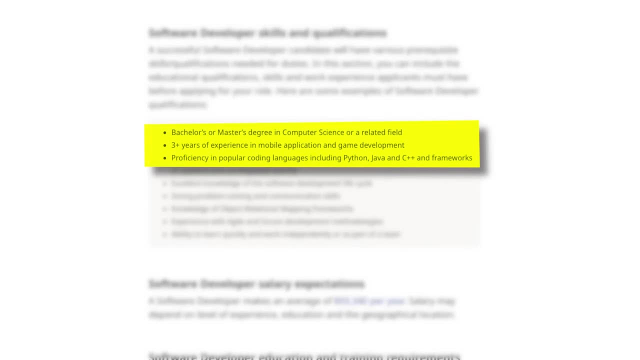 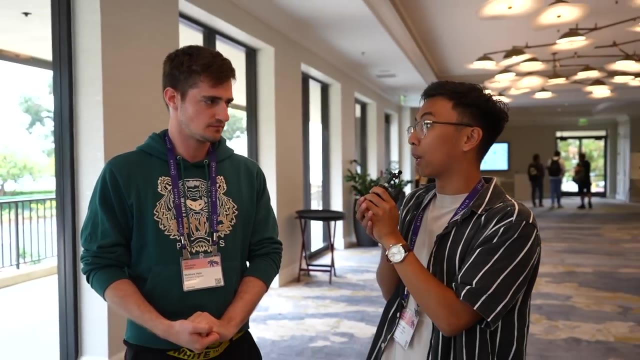 Even if it doesn't, If I don't have the years of experience, If I don't meet every single qualification, I would say: go for it. Like the worst that can happen is they say, no, Awesome. Okay, And when you got your first job as a developer, how much did you make?